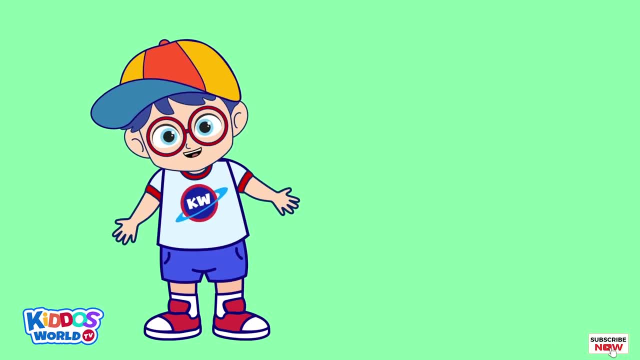 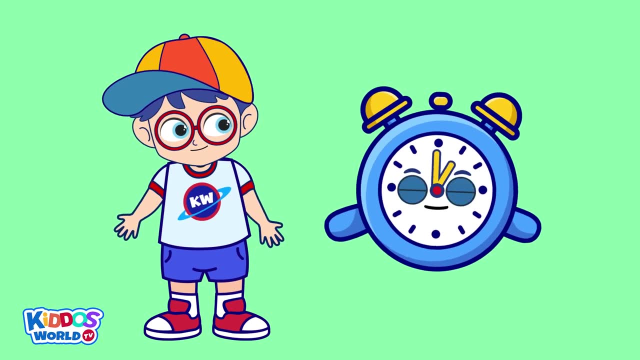 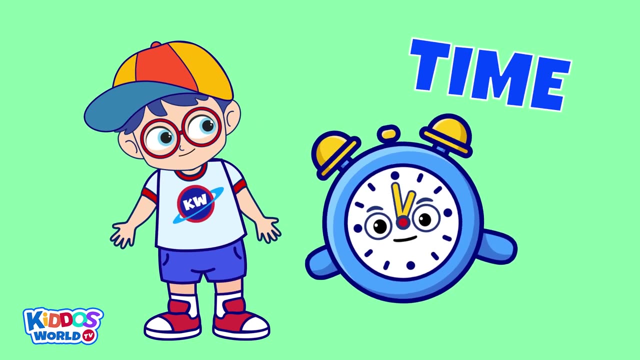 And to help us with this task, let me introduce to you my trusty friend Clocko. Hello kiddos, As you can see, I am a clock And today I'm going to teach you how to read time. But first let me show you my parts. 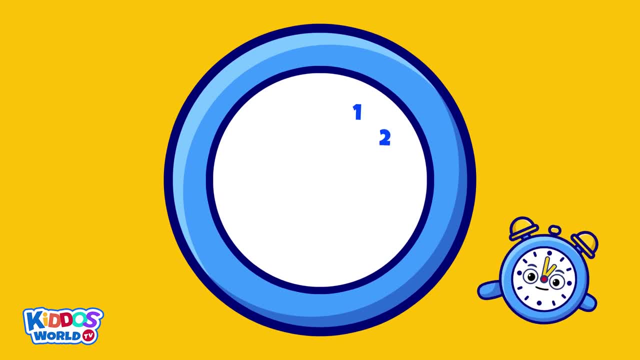 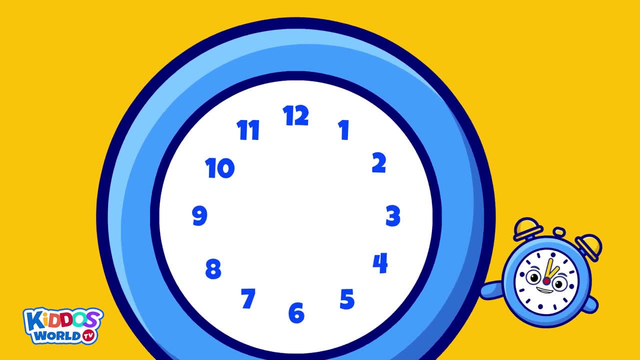 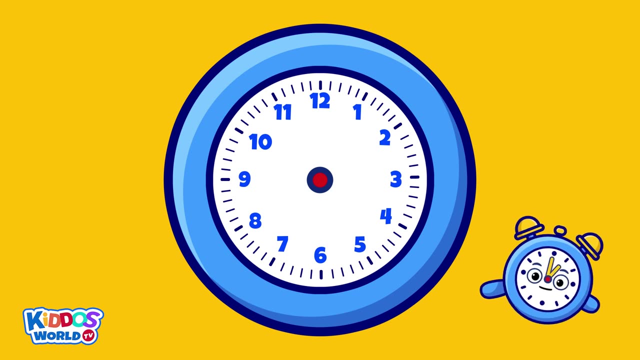 My face has numbers that run from number 1 up to number 12!. It also has five lines between numbers. Now let's proceed to my two most important parts, which are my hands: My big hand and my small hand. My small hand shows the hour. 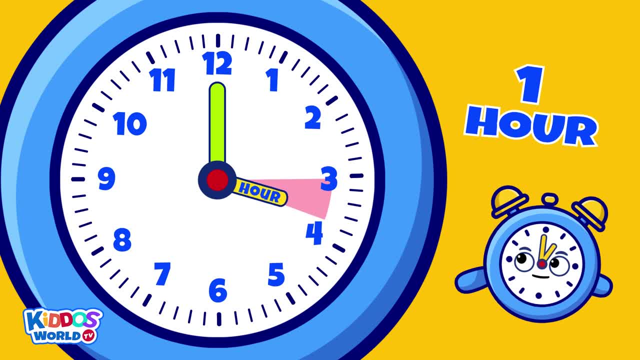 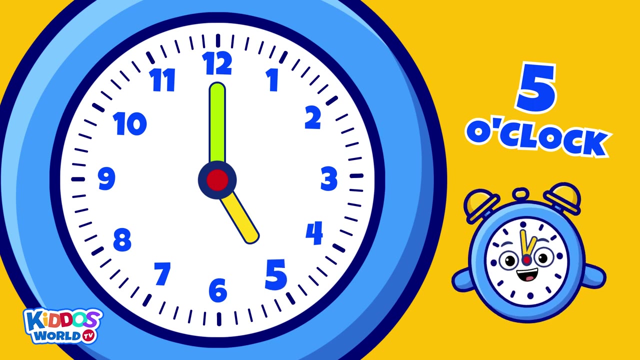 Every time my small hand moves from one number to the other, it means one hour has passed. For example, when my small hand pointed at number 1, moves to number 2, we read the time as 2 o'clock. When it moves to the number 3, it's 3 o'clock, and then it moves again. now it's 4 o'clock, 5 o'clock, and so on. 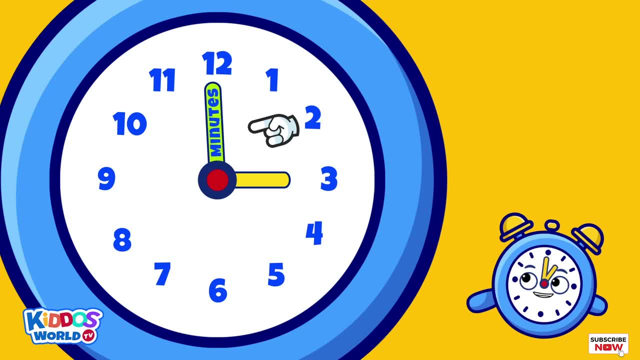 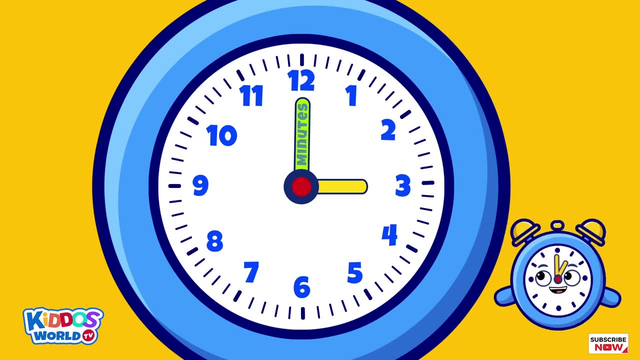 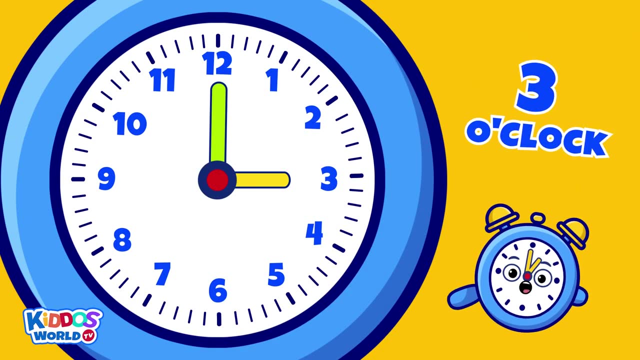 Meanwhile, my big hand shows the minutes. Now look closely as I show you a total of 60 small lines around my face. These lines represent 60 minutes in an hour. For example, it's 3 o'clock. Now look closely as my big hand makes a movement and landed in the first small line. 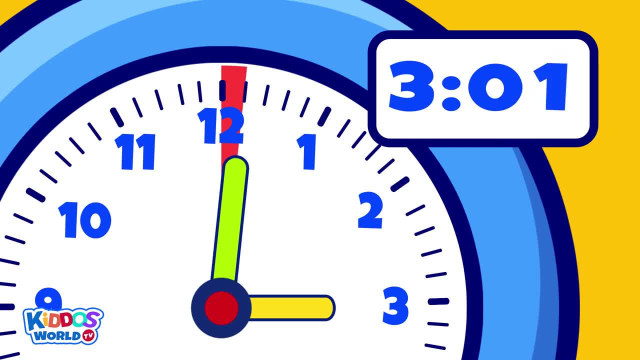 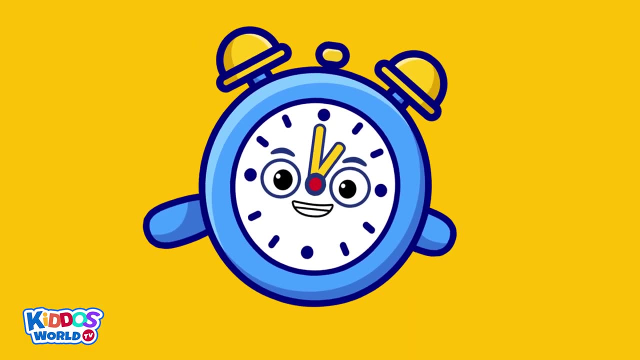 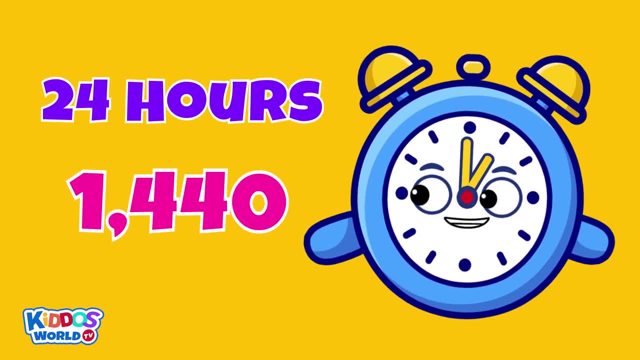 There are 24 hours or 1,400 minutes. There are 24 hours or 1,400 minutes, And reading the time in a clock can help us easily distinguish day from night. And reading the time in a clock can help us easily distinguish day from night. 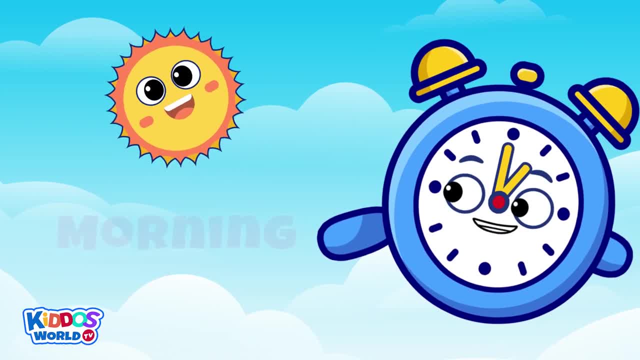 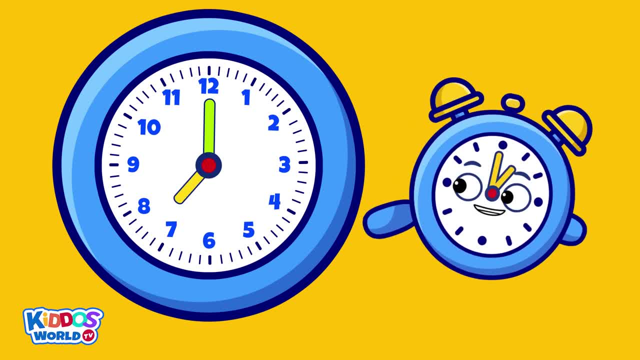 When my small hand made a full movement in my face, it means 12 hours has already passed. When my small hand made a full movement in my face, it means 12 hours has already passed. It's the afternoon, or a new day has begun. 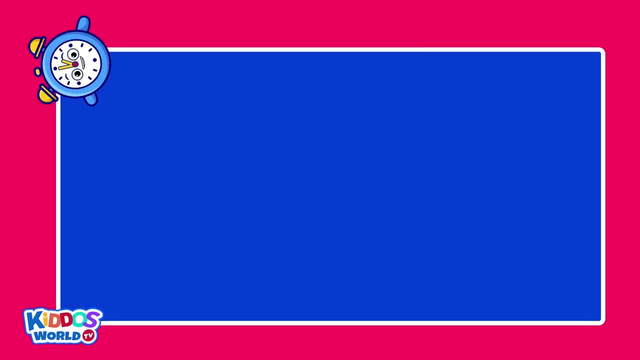 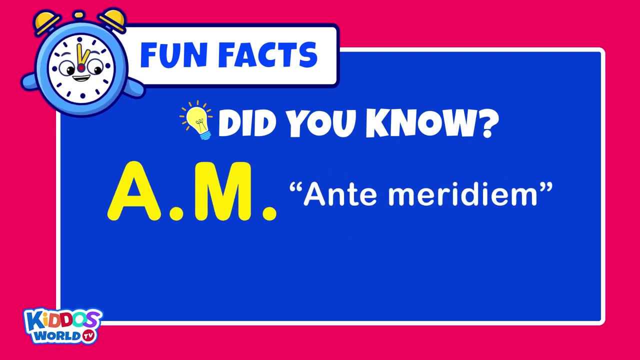 It's the afternoon or a new day has begun. Here are some kiddo's fun facts. Here are some kiddo's fun facts. Did you know that AM is short for the Latin phrase anti-meridiem, which means before midday or before noon? 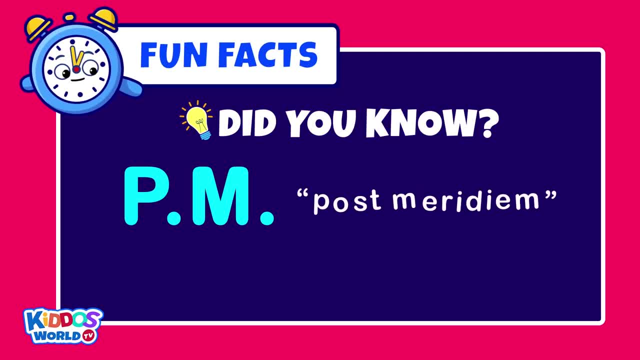 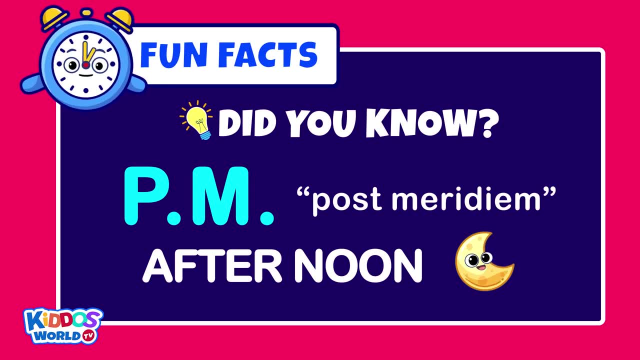 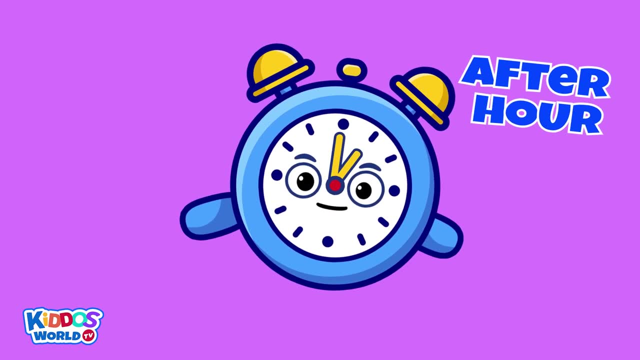 Meanwhile. PM stands for the Latin phrase post-meridiem, which means afternoon or after midday. Now let's practice. For now, let's guess the time after the hour. Are you ready? Here we go. Can you tell me the time? 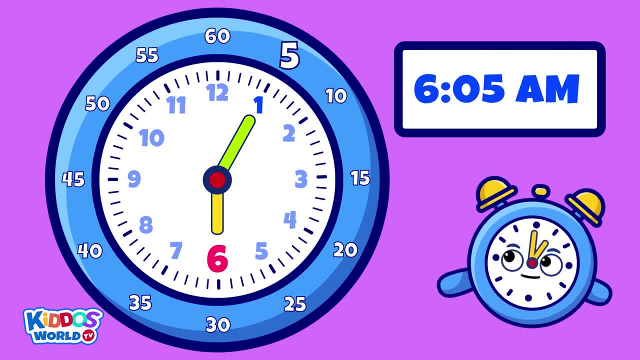 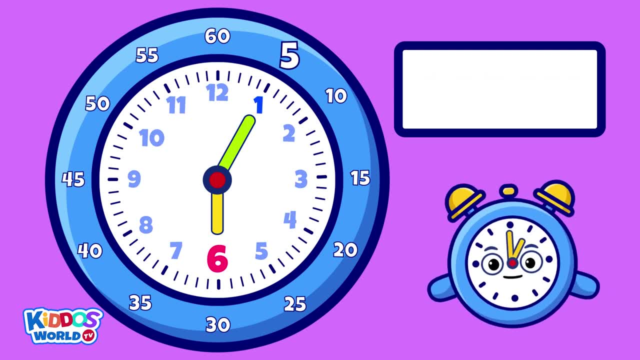 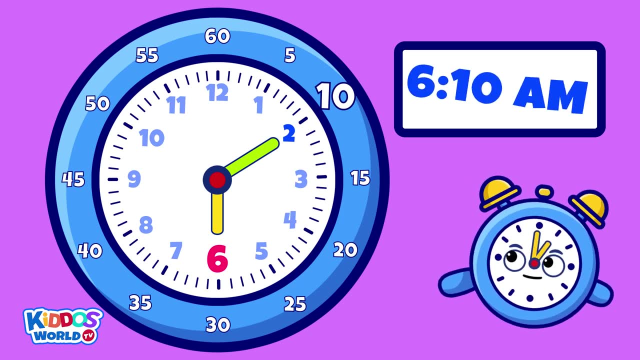 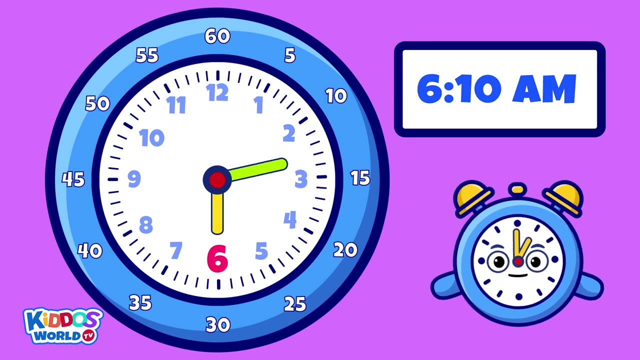 That's correct. It's five past 6 am or 6.05 am. How about this time? Yes, It's 10 past 6 am or 6.10 am, And this one You're absolutely right. 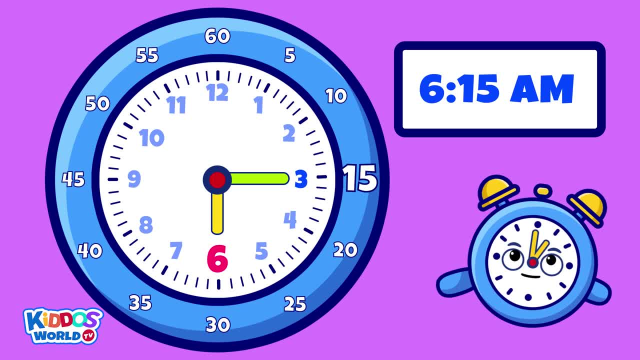 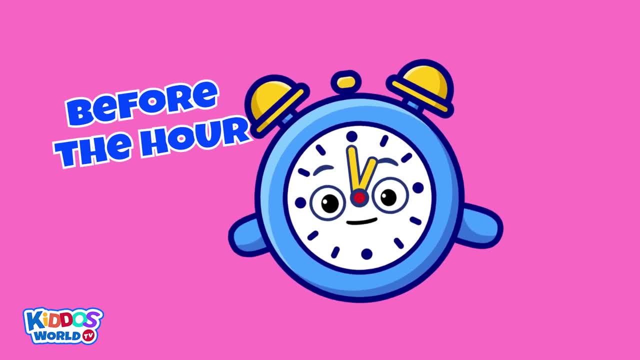 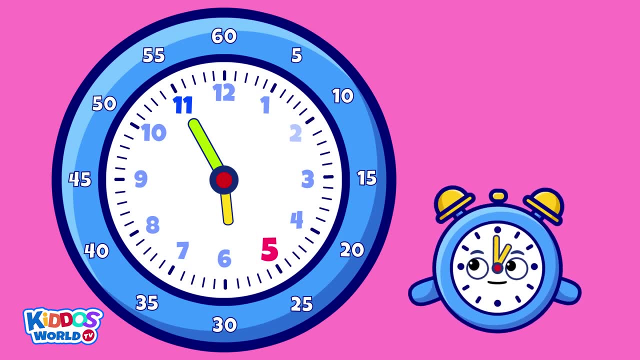 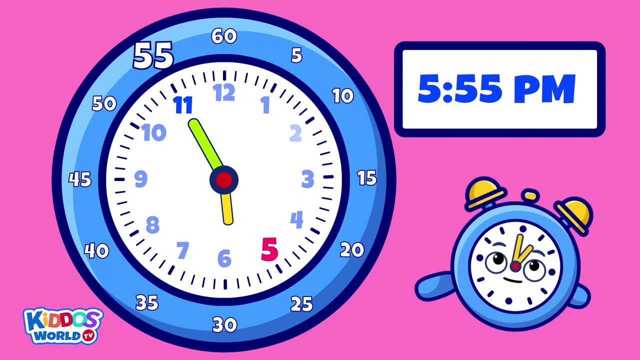 It's 15 past 6 am or 6.15 am. We can also tell time before the hour. Kiddos, can you tell me the time Correct? It's five before 6 am or 5.55 pm. 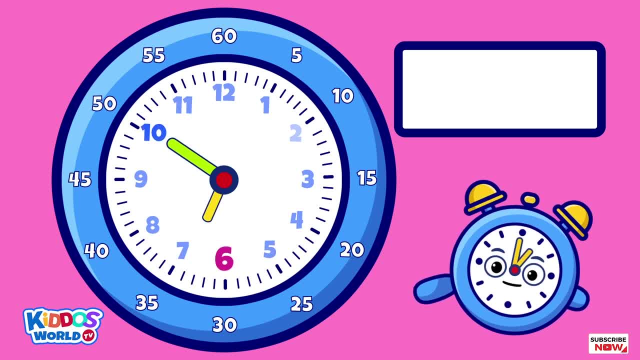 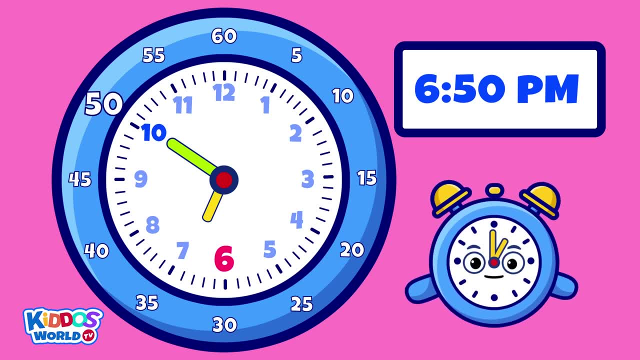 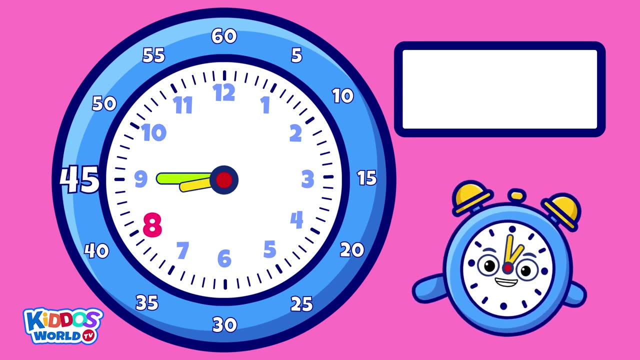 Let's try another one. It's 10 before 7 pm or 6.50 pm. How about this one, Fantastic. It's 15 to 9 pm or 8.45 pm, Yay. 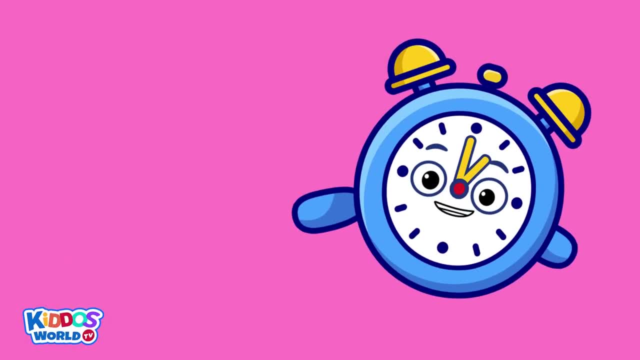 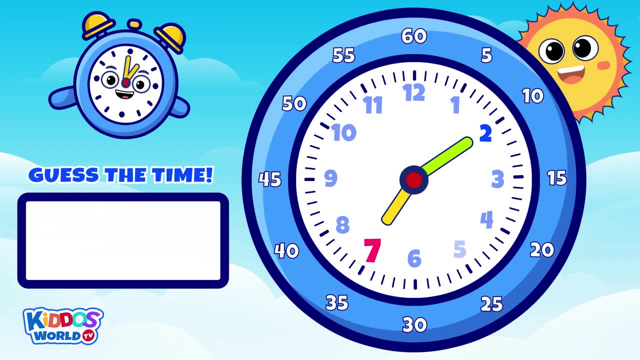 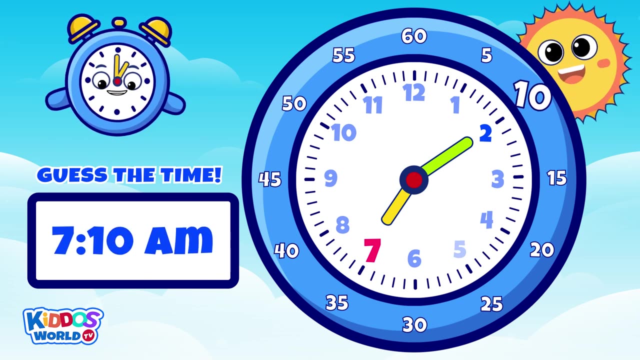 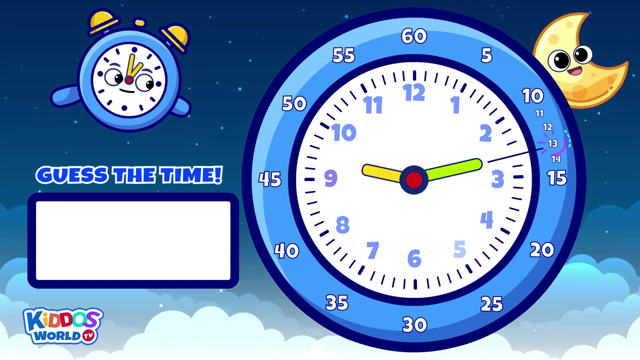 Are you still game for another exercise? Let's do it. Kiddos, can you tell me the time? Correct, It's 7.10 am. Let's do another one. That's right, It's 9.13 pm.